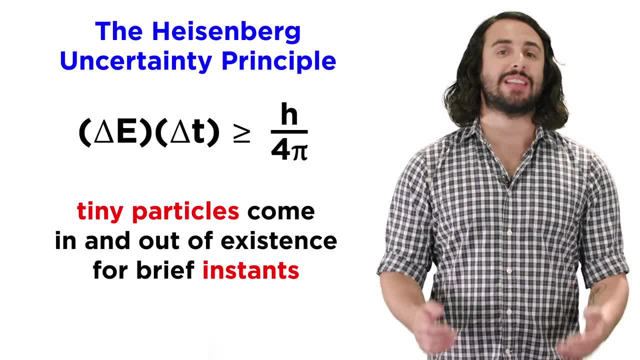 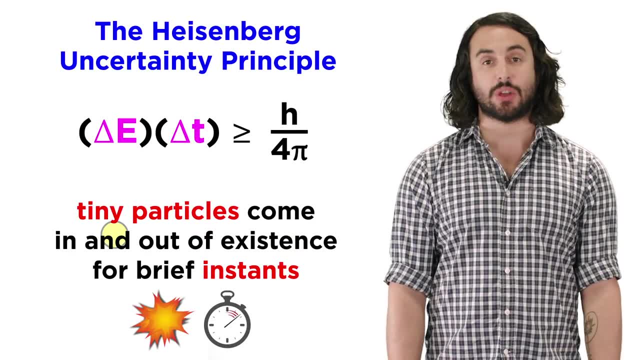 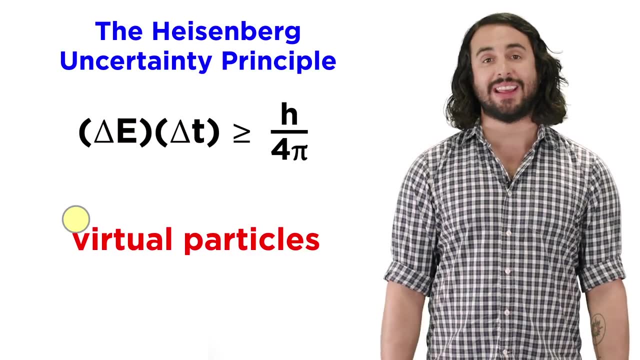 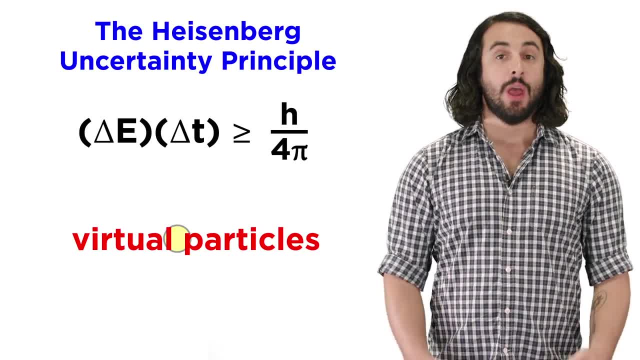 particles that make up ordinary matter. 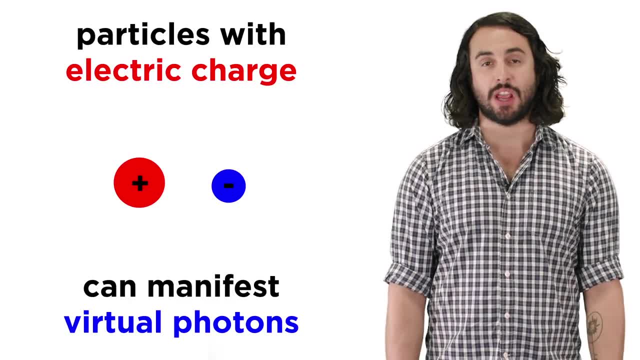 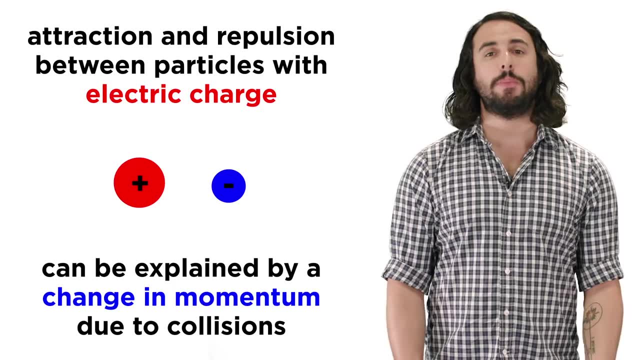 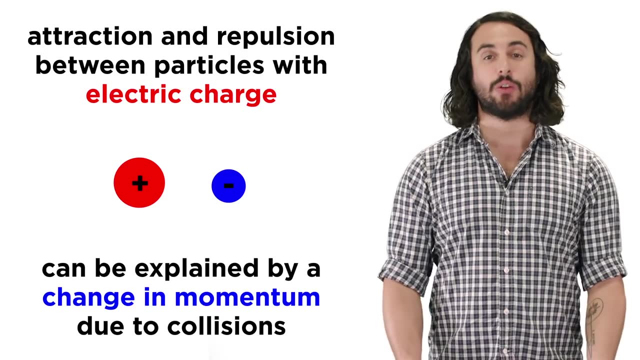 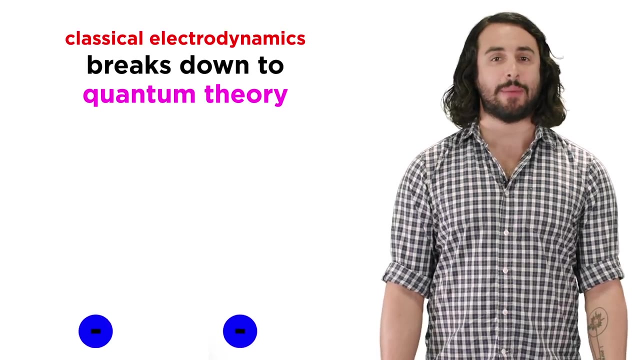 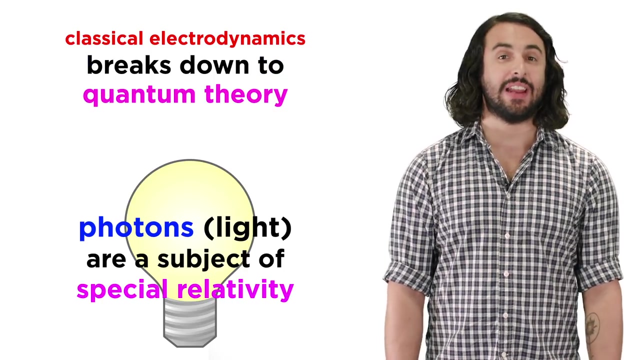 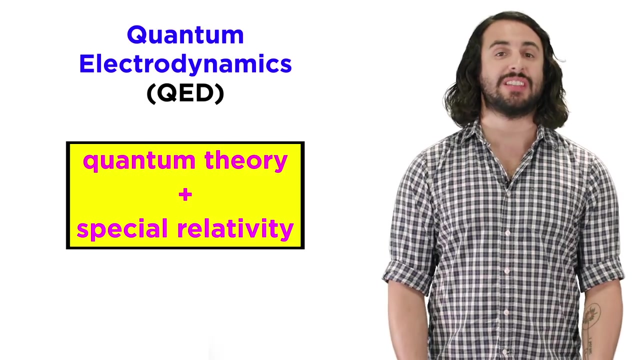 But if it were the case that charged particles like protons and electrons were able to manifest these virtual photons, then the attraction and repulsion between charged particles would be explained by the exchange in momentum that occurs during collisions between virtual photons and regular particles. No electromagnetic field would have to be referenced. This means that classical electrodynamics can be explained by quanta, and therefore quantum mechanical principles. And since light is a subject of special relativity, this makes QED a successful merging between special relativity and quantum theory. 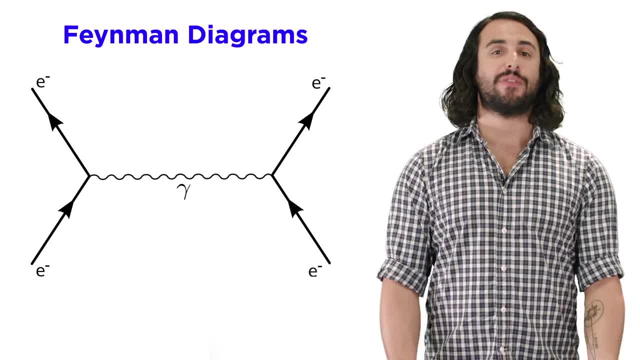 To illustrate the exchange of virtual particles, Feynman developed a system for representing 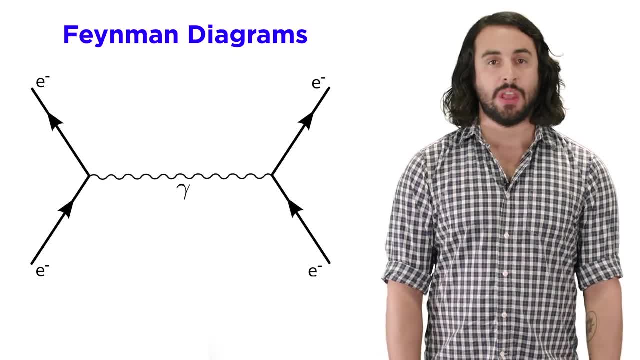 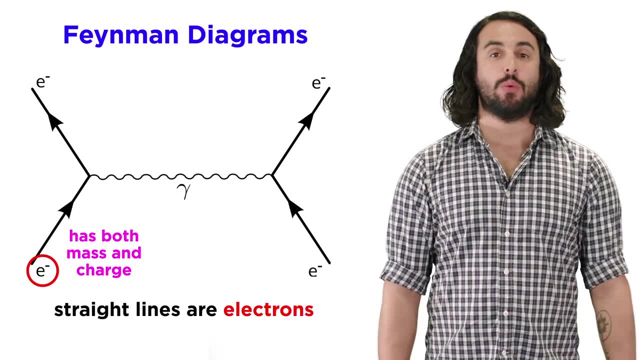 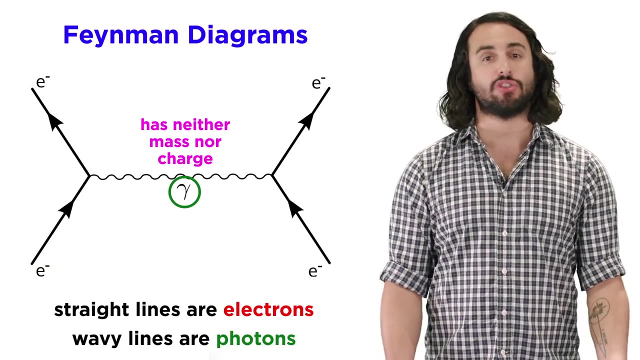 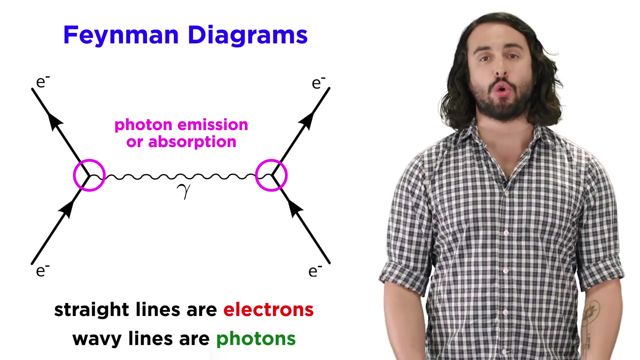 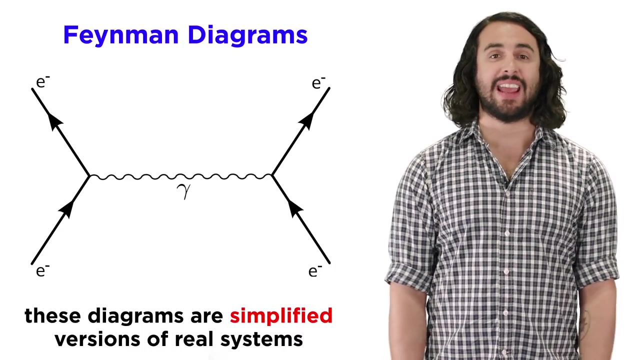 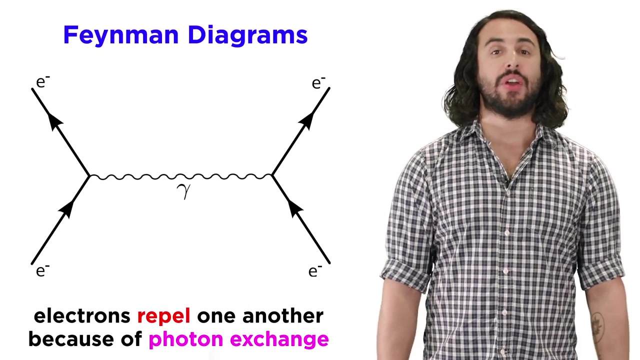 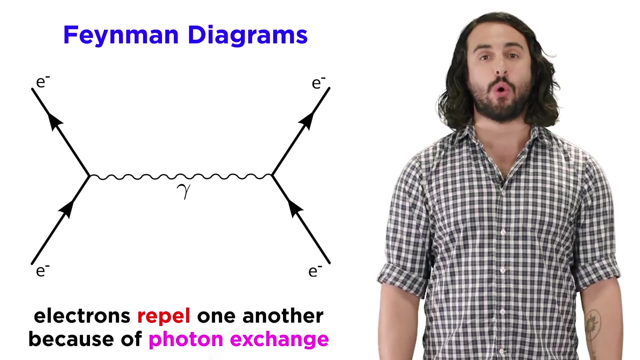 quantum phenomena called Feynman diagrams. In these surprisingly simplistic representations, a straight line signifies an electron, which we know has both mass and charge. A wavy line signifies a photon, which has neither mass nor charge, and when there is a junction between a straight line and a wavy line, this means that the electron has either absorbed or emitted a virtual photon. These diagrams are mere reductions of reality, they do not contain all the information that could be pertinent to a system of one or more electrons, but they illustrate in a basic way that two electrons could approach one another and then have their paths deflected due to the exchange of one or more virtual photons that carry some momentum. 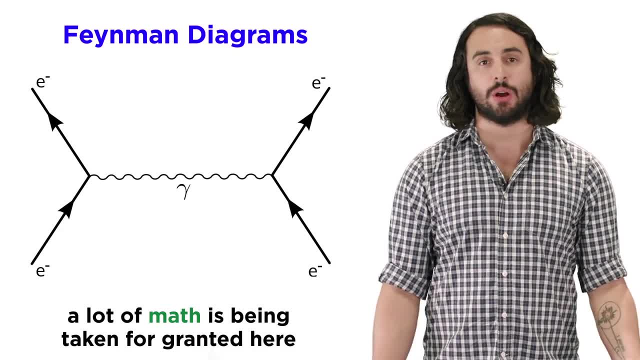 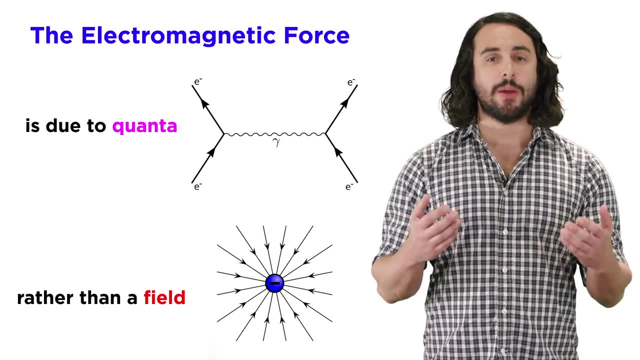 Given that this is quantum mechanics, there is a ton of math we are glossing over, but the main takeaway is that the electromagnetic force has been demonstrated to be the result of particle exchange, or quanta, rather than an electromagnetic field. 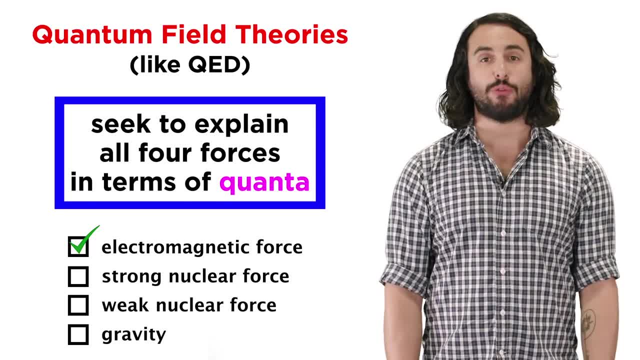 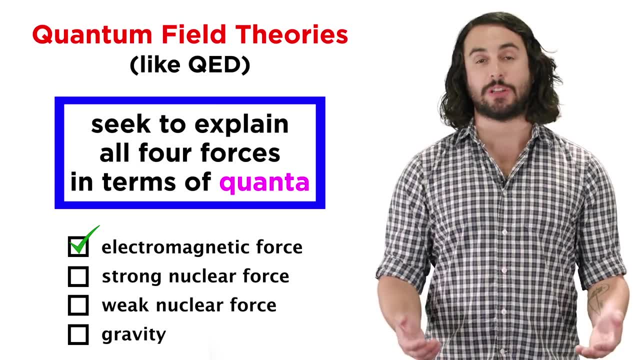 Quantum field theories, such as QED, seek to explain all four fundamental forces in this regard, and they have been largely successful, so let's move forward and see which force was to be updated next.